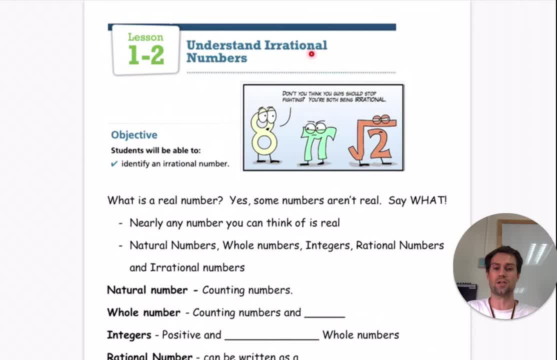 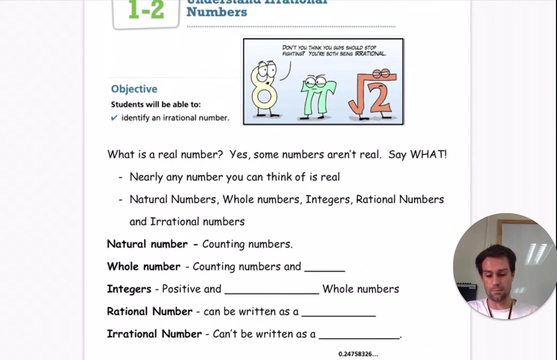 But for 1-2, we're going to be looking at irrational numbers and we're going to be understanding what an irrational number is. We will also be looking at what real numbers are and how we can classify those on the number system. So our objective is: we are going to identify an irrational number. So an irrational number is a real number. So we have irrational numbers. Those are real numbers. Now you might say to yourself: a real number, Does that mean there are fake numbers? Well, actually there are. There are numbers that are called 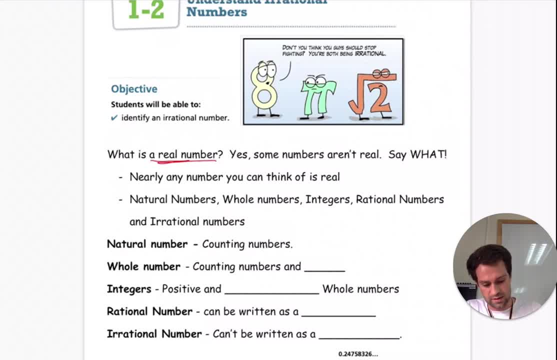 imaginary numbers And those numbers, for example, would be: the square root of negative. 1 is an example of an imaginary number. And another example would be: infinitely would not be an imaginary number, but that is an idea. So square root of negative 1, should put this over here- square root of negative 1.. This is imaginary. 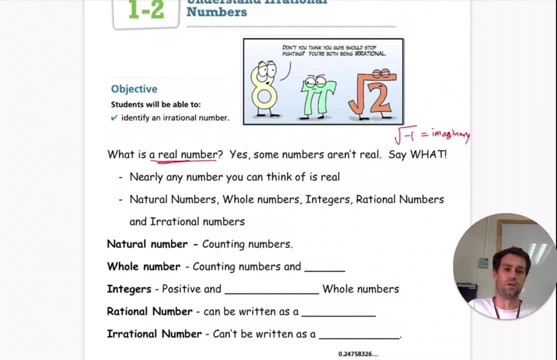 Okay, and we're not going to be looking at imaginary numbers. That is something that you'll be covering once you're in high school. So, basically, any number that you can think of is a real number and we can classify those real numbers as a natural number, as a whole number, as an integer, as a rational number. 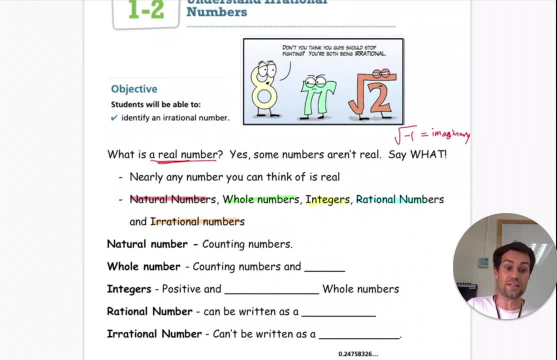 And, as an irrational number, numbers. So we have five different types of numbers here. So a natural number is a counting number, a number that you can count. So, for example, one, two, three, four, five, those are all. 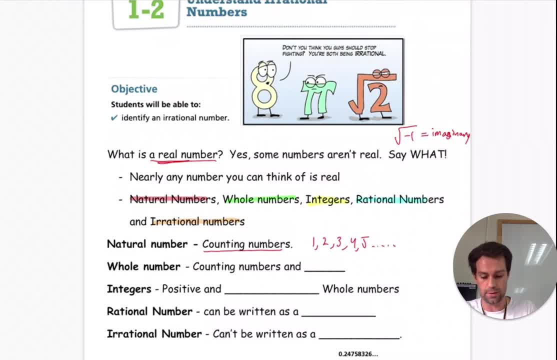 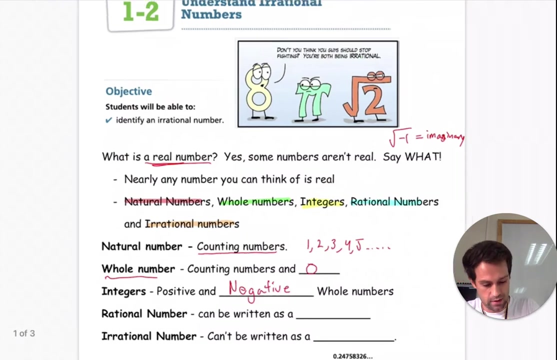 natural numbers. A whole number, a whole number is a counting number, and zero, Zero is also a whole number. So a whole number, zero is not a natural number, but just a whole number. Integers are positive and negative whole numbers, So we could have negative three, negative two. 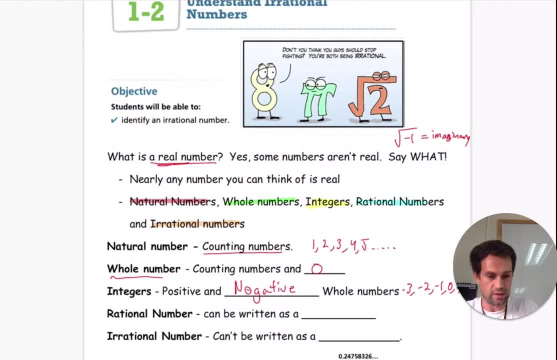 negative, one, zero, one, two. It keeps on going. Okay, Negative and positive. Oh, you can't see that. You can't see that because of my lovely face there. We'll move that up. Okay, Rational number can be written as a fraction. Okay, So a rational number can be written as a fraction. 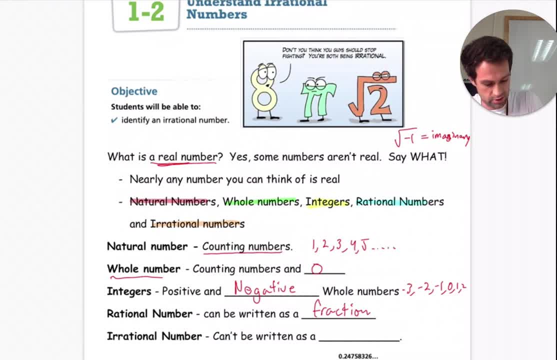 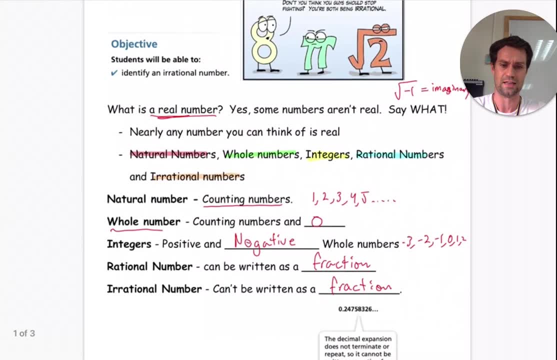 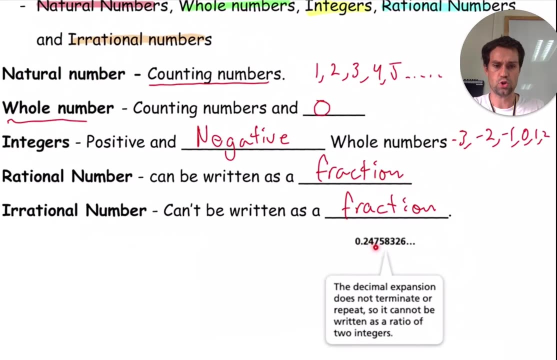 An irrational number cannot be written as a fraction. Okay, And we'll be looking at this. So you probably will have to pause the video here so you can get these notes down. So we have, uh, this number here is 0.24758326: dot, dot, dot. This means it keeps going forever. 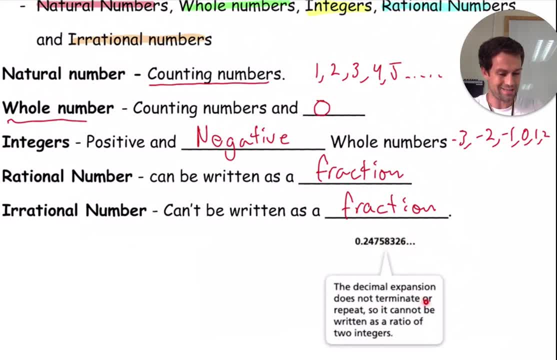 The decimal expansion does not terminate, It does not stop, It does not or repeat, It does not repeat. It just keeps on going forever. So we cannot write this as a ratio. That's a fancy way of saying. we cannot write this as a fraction. 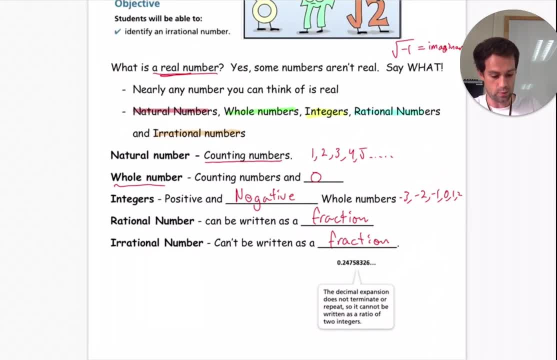 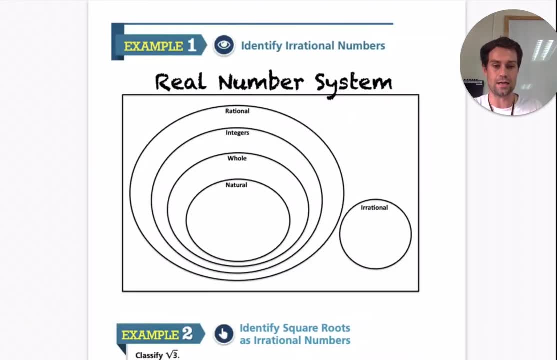 So this is a irrational number. So we're going to go ahead and classify these numbers on the number system. So we have our natural numbers here. Okay, The natural numbers. I'm actually not going to highlight that. The natural numbers we said are one, two, three. 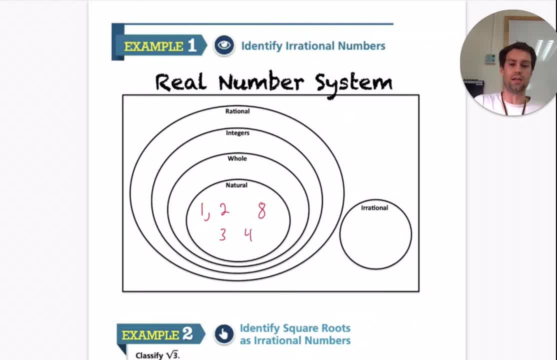 four, eight. These are all natural numbers And all of these natural numbers are whole numbers. All of these numbers, this in this Venn diagram, anything that falls into this category here falls into the whole number category. There is one number that is a whole number, that's. 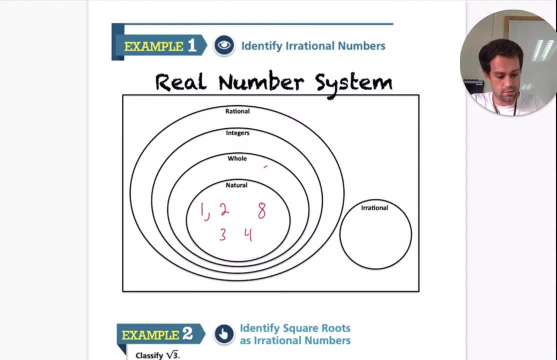 not a natural number. Zero. We talked about that earlier. Zero is a natural number. Zero is a natural number. Zero is a whole number. Now, all of these whole numbers are integers, but there's other numbers up here that are not. 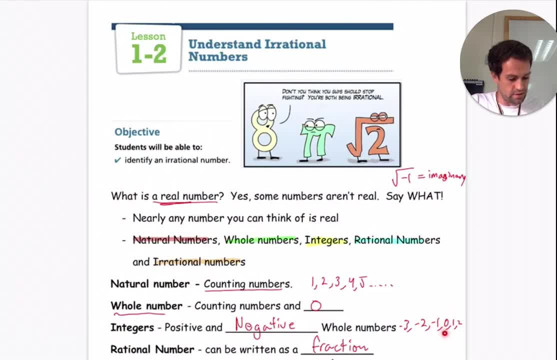 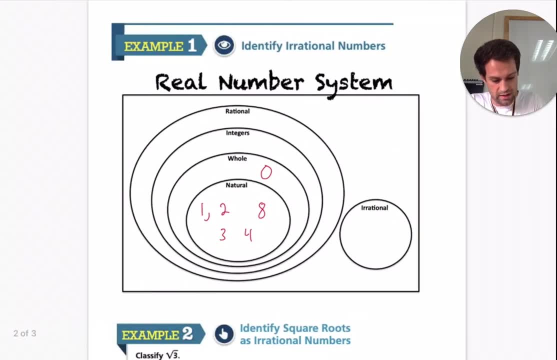 integers, meaning here All of these numbers. here were whole numbers, but our integers can also be the negative numbers. So negative eight negative two negative one negative 100.. These are all integers. I could write five as an integer. However, five is also a whole number and five is also a natural number, So there is no reason to write five as an integer or a whole number. 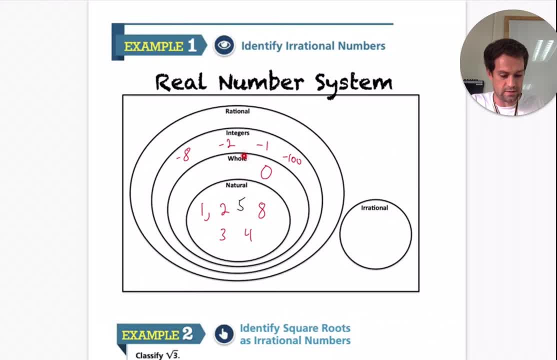 We can write it as a natural number because it falls into these other categories. So a rational number could be negative: four over five, two over three, zero point one, five. That is a rational number because we can write it as a fraction: One over two. zero point six, six, repeating. because zero point six, six repeating is the same as two over three. 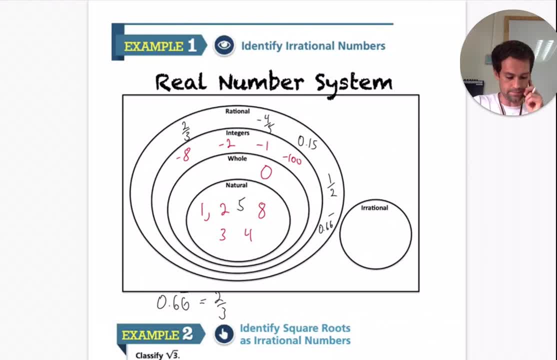 So those are all rational numbers, OK, An irrational number would be a number that does not terminate. So zero point. One, two, one, two, two, one, two, two, two keeps going. There's no pattern. It keeps adding. 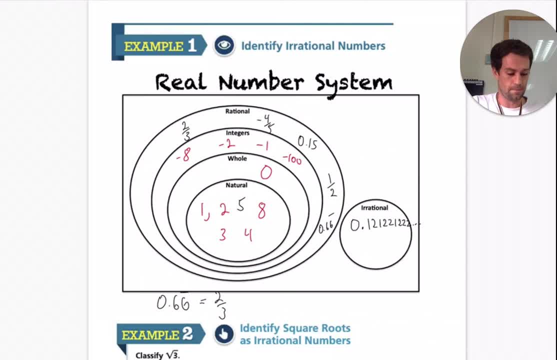 We cannot write that as a fraction. The most popular people would say: irrational number is: is Pi, Pi is an irrational number. Or we would have the square root of two or the square root of three. These are all irrational numbers. 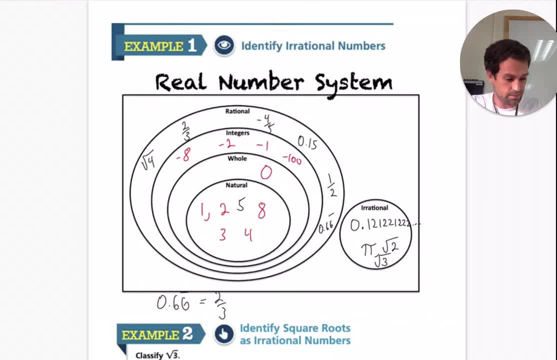 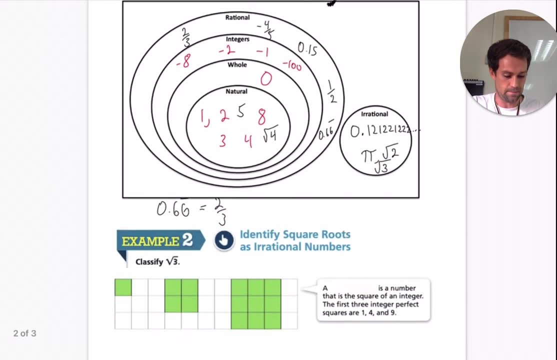 Square root of 4 is actually 2.. So the square root of 4 is 2, so that would actually be a natural number. Okay, so a little bit of classification there. So let's classify the square root of 3.. 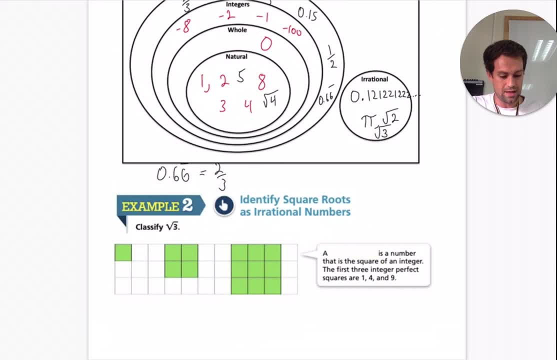 So we saw that the square root of 3 is irrational. Let's look at this in a diagram to understand this a little bit more. So a perfect square is a number that is the square of an integer. The first three integer perfect squares are 1,, 4, and 9.. 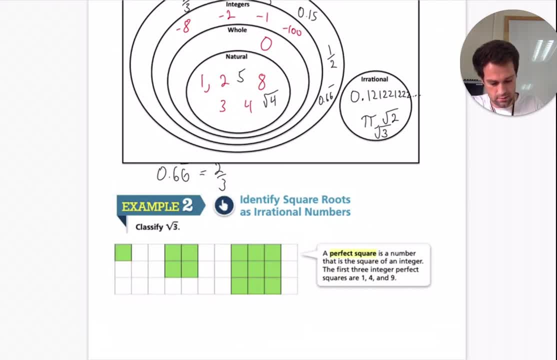 So we can see, this is 1,, this is 4, and this is 9, meaning square root of 1, the square root of 4, and the square root of 9.. The square root of 1 is 1 times 1.. 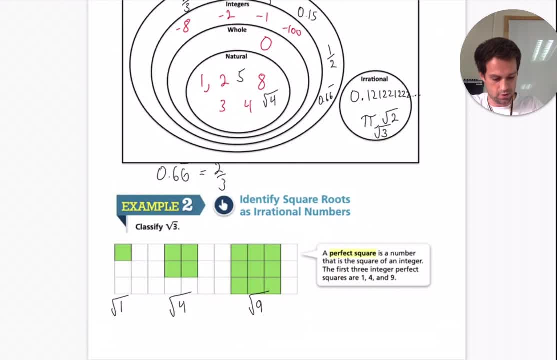 So 1 times 1 equals 1, or 2 times 2 equals 4, or 3 times 3 equals 9,. right, The square root of 1 is 1,, the square root of 4 is 2,, the square root of 9 is 3.. 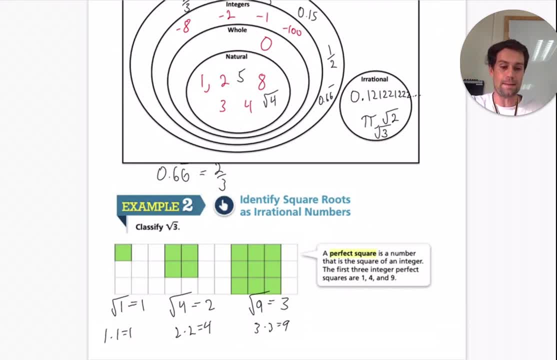 Well, the square root of 3 is not a perfect square, so it does not repeat, and we cannot write that as a fraction. So the square root of 3 is not a perfect square, so it does not repeat, so the square root of 3 is irrational. 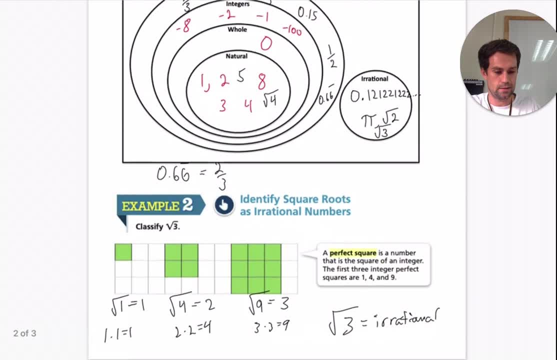 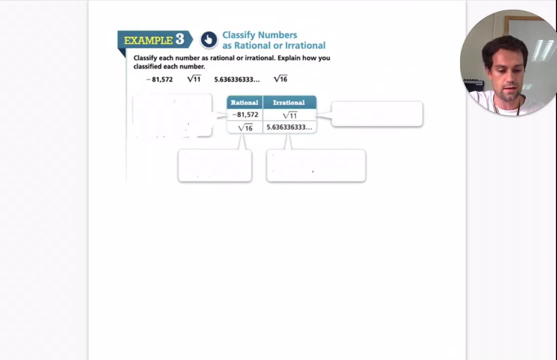 Okay, And this is the last bit that we will cover. The video is getting a little bit long. I apologize for that. So we want to classify each number as a rational or irrational and explain how you classify these numbers. So we're classifying these four numbers here. 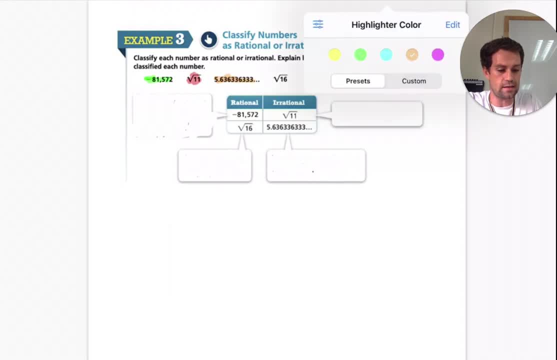 and they organize this in the table. okay, So the negative 81,572 is an integer, because it can be written as a fraction over 1.. The square root of 16 is a rational number, because the square root of 16 is 4.. 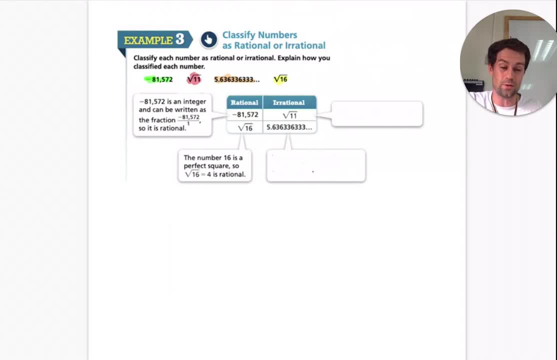 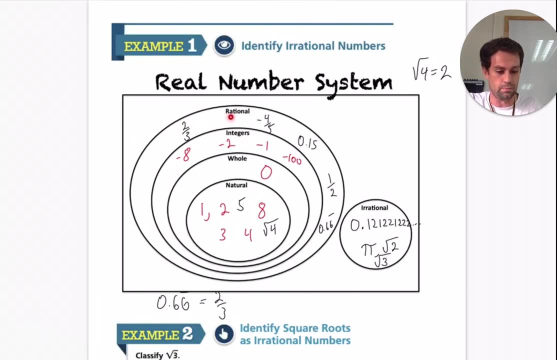 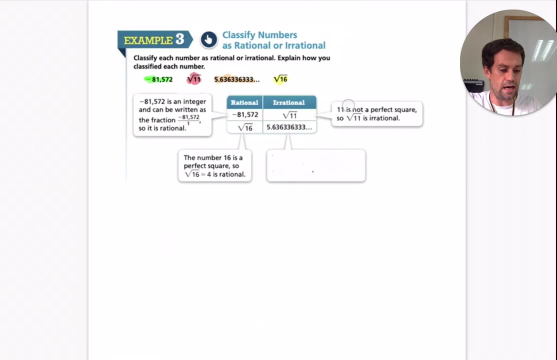 The square root of 16 is 4.. 4 is irrational Number 4 is actually a natural number as well. right, It goes here, It is rational, but it's an integer, all and it is natural. The square root of 11 cannot be written as a perfect square. 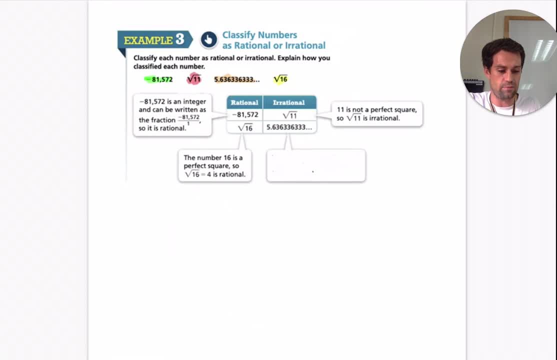 so it is irrational. And 5.6363363333.. keeps going cannot be expanded as a fraction. The decimal is non-terminating, So it is not repeating, so it is irrational. okay, Please write down any questions that you may have. 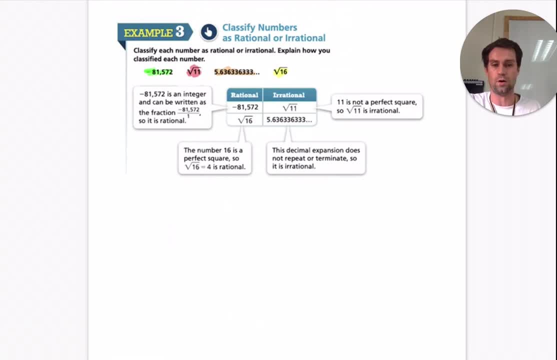 Make sure you got this written down in your notebook And have a wonderful day.